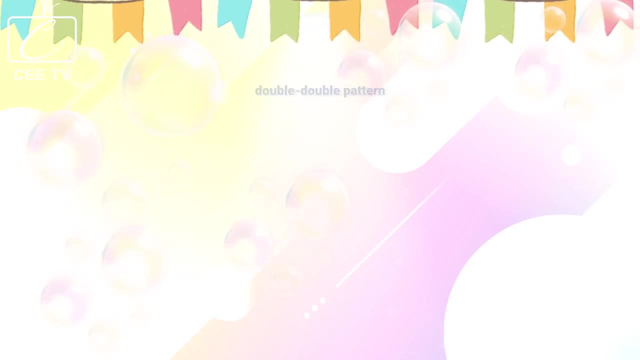 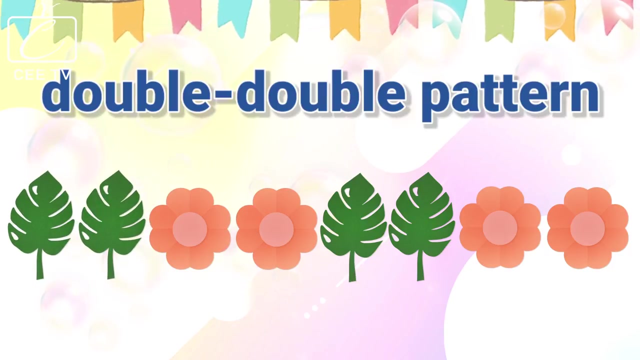 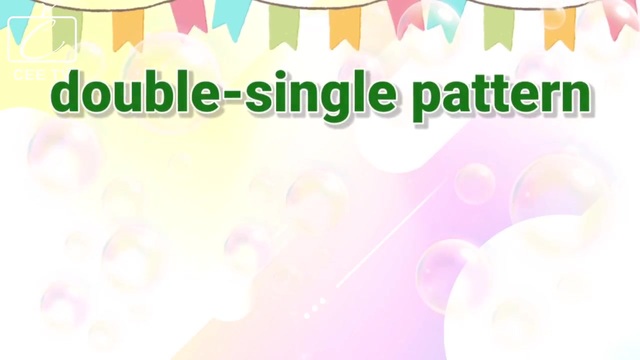 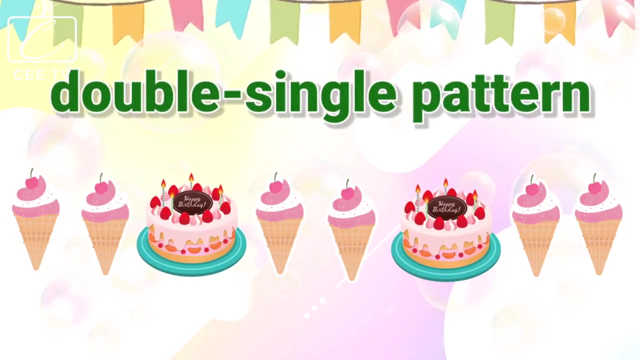 A set of objects can be arranged in a double-double pattern. We have here a leaf, another leaf, a flower, another flower. A set of objects can also be arranged in a double-single pattern. We have here an ice cream, another ice cream, a cake, an ice cream, another ice cream, a cake, an ice cream and a cake. 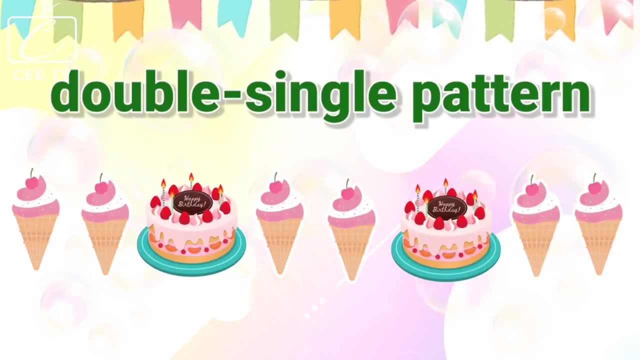 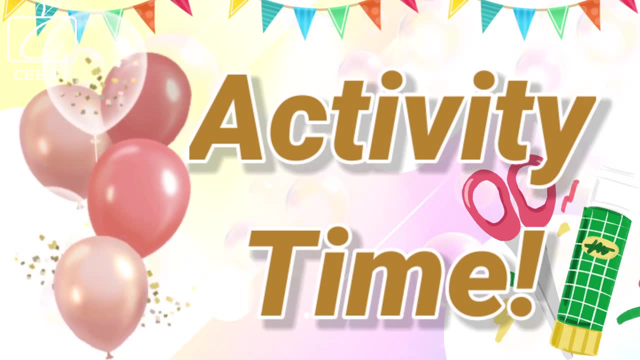 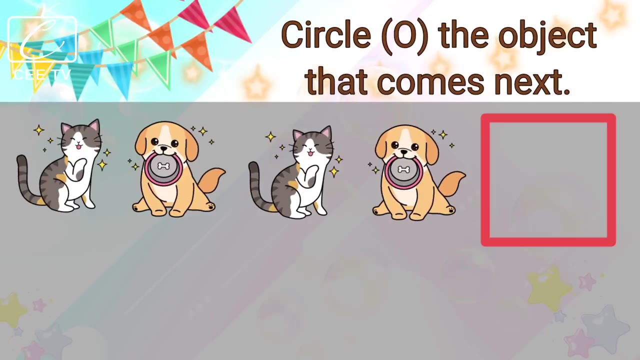 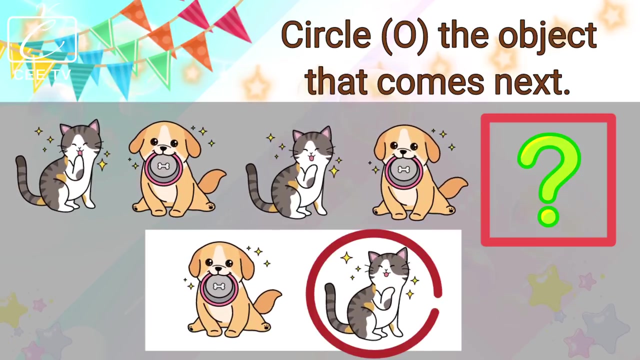 A cake, an ice cream and another ice cream. Activity Time Circle: the object that comes next: A cat, a dog, a cat, a dog. what comes next? Is it the dog Or The cat? The cat comes next. 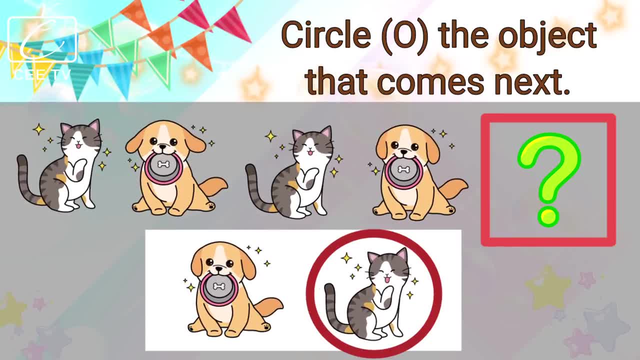 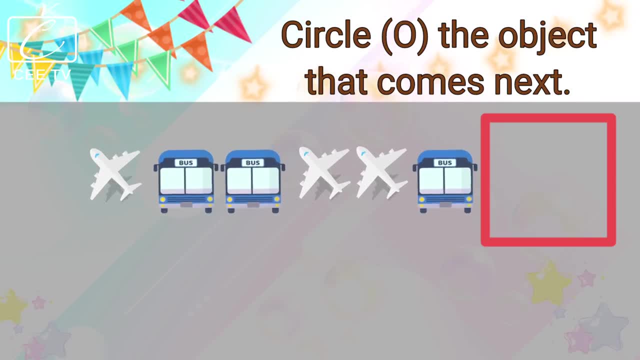 You are right, The cat comes next. We have here An airplane, Another airplane, A bus, Another bus. An airplane, Another airplane, A bus. What comes next? Is it the bus or the airplane? The bus comes next. 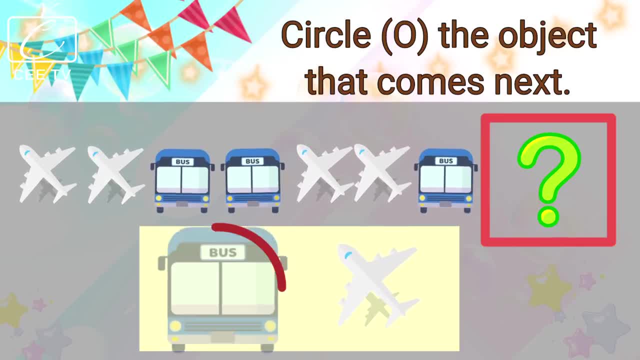 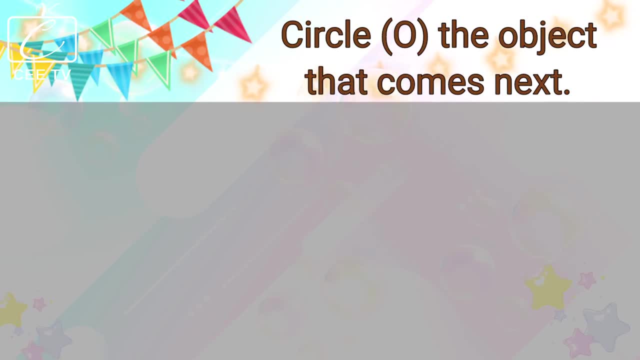 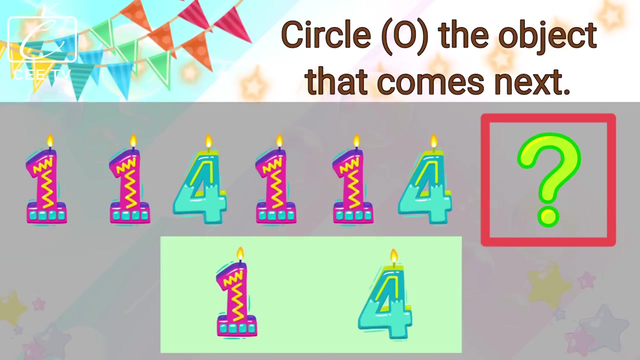 Great job, You are correct. The bus comes next. We have here A number one candle, Another number one candle, A number four candle. A number one candle, Another number one candle, A number four candle. What comes next? Is it the number one candle or the number four candle? 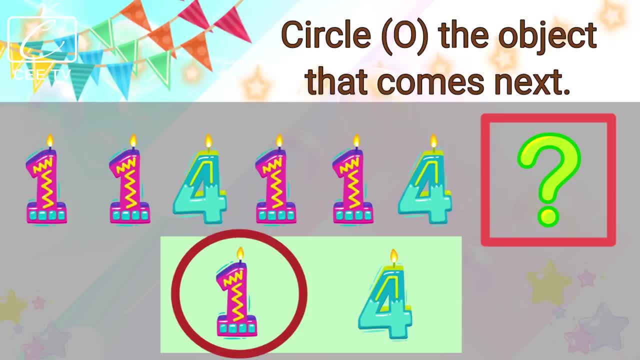 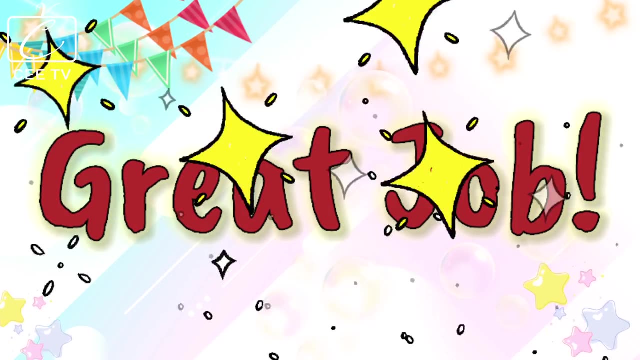 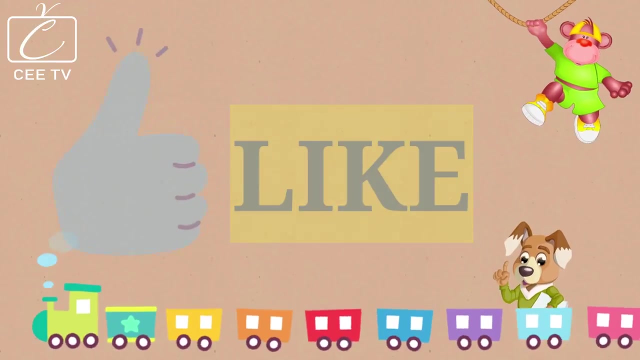 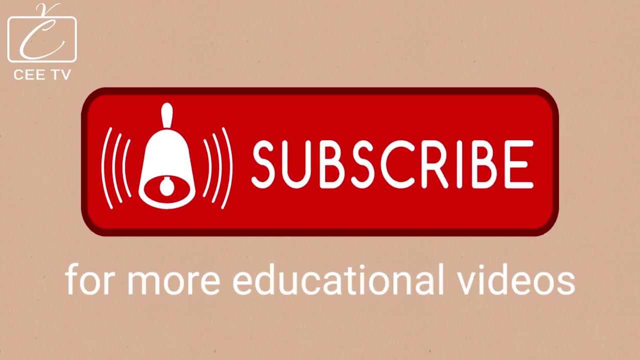 The number one candle comes next. Excellent, You are correct, The number one candle comes next. You did a great job. Thank you for watching. If you like our video, please press the like button and share it with your friends. We will be posting more educational videos. 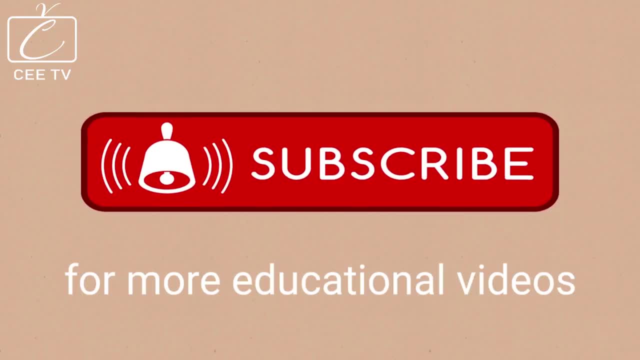 Don't forget to subscribe. See you in our next video.